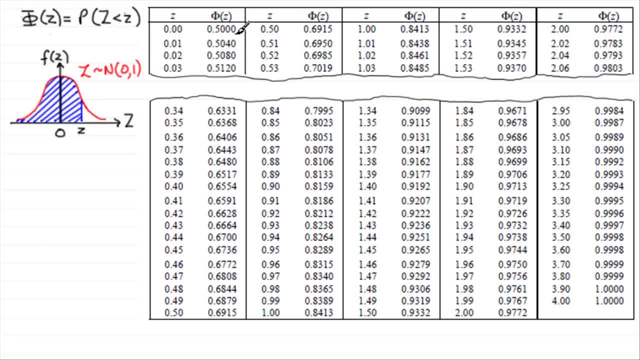 So you can see that phi of Z is 0.5.. You'll also notice that if you go to Z being 3, three standard deviations above the mean, then we have a probability here of being less than 3 standard deviations of 0.9987.. 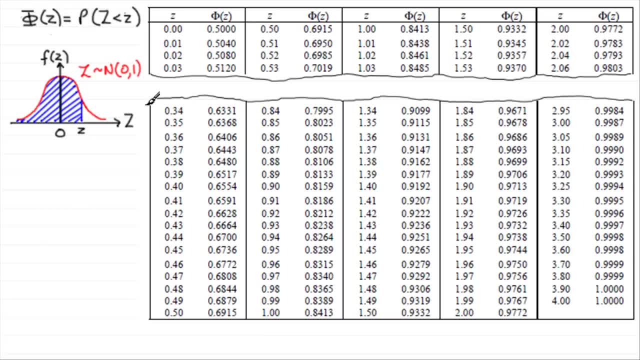 Almost 1, almost 100%. So if you went 3 standard deviations up here, you'd have nearly shaded the whole lot. Now, suppose, then, that you had to work out this probability here, the probability of Z being 1.2. 1.5. What I would need to do, then, is work out what phi of 1.5 was. You don't have to. 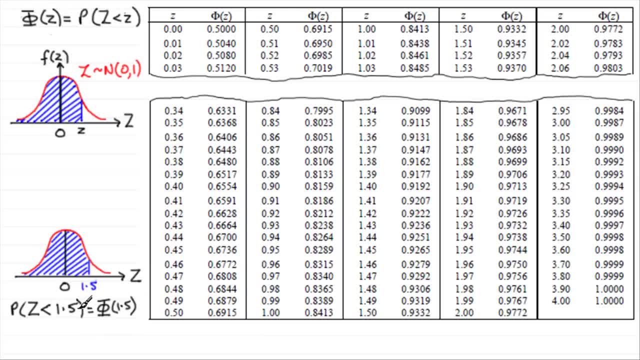 write that some people don't. they just live with this. so that's fine. But what is it? Well, it's going to be found in this section of the tables. I'll just put that section down here, ok. And so when we look up 1.5, it's clearly this value in here: 0.9332.. So 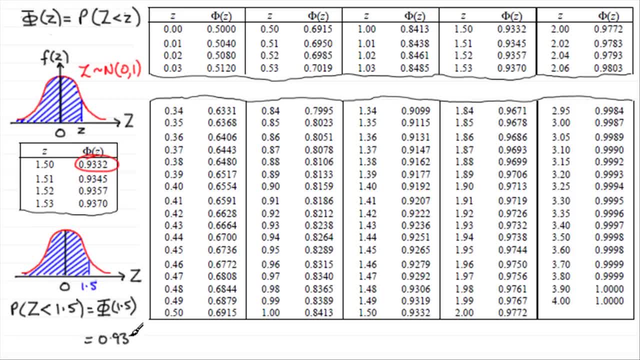 the probability would be 0.9332.. Now, what I want to show you now, though, is how to work out other probabilities of being greater than, or less than, or more than, particular values. Why? because these tables are restricted. They've got our z values that go from 0 to 4 standard. 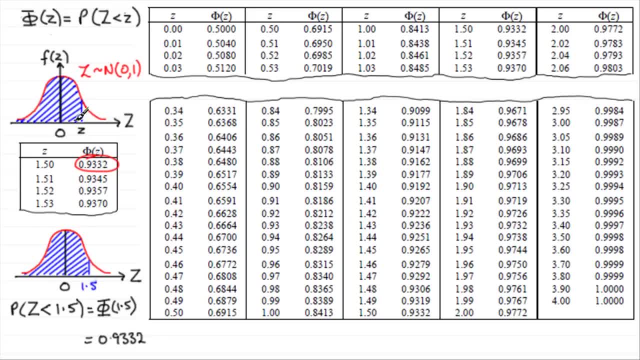 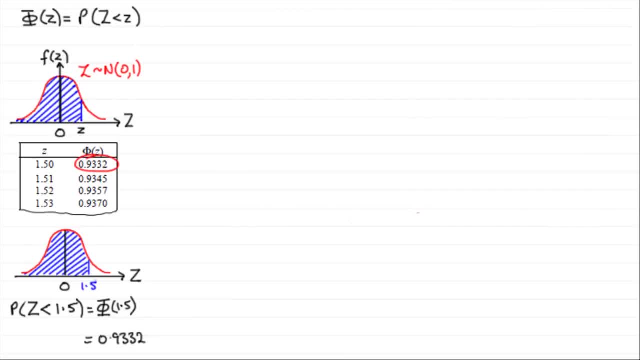 deviations, That is, they're to the right of 0 and only give us the area to the left of z. Now suppose we had to work out the probability of z being more than 1.5 standard deviations from the mean. Well, to do this, our tables, as I say, only give us area to the left. So to get around, 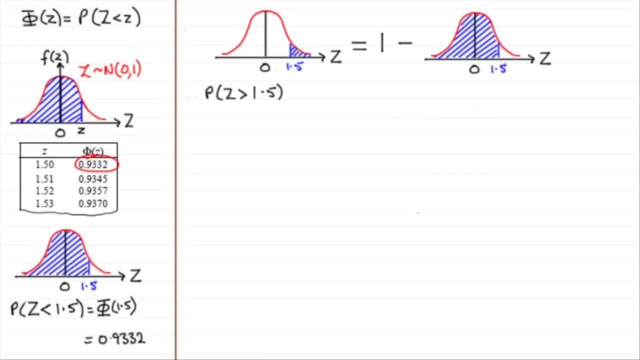 this problem. what we do is we look at the area under the whole graph, which would be 1, and take away the area to the left of 1.5. So all we need to do is 1 minus the probability of z being less than 1.5, or phi of 1.5.. 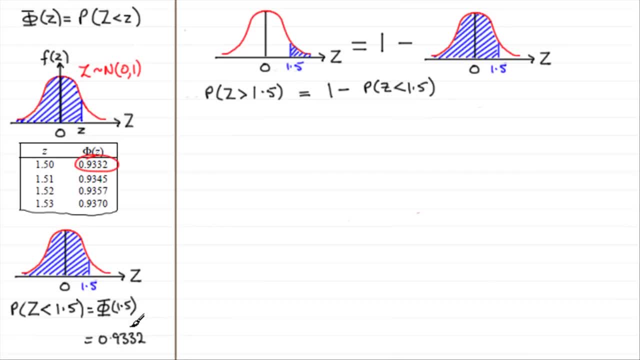 So we take away the area to the left of 1.5.. So we take away the area to the left of 1.5.. And we've got that down here: 0.9332.. So we've got 1 minus 0.9332, and that comes to 0.0668.. 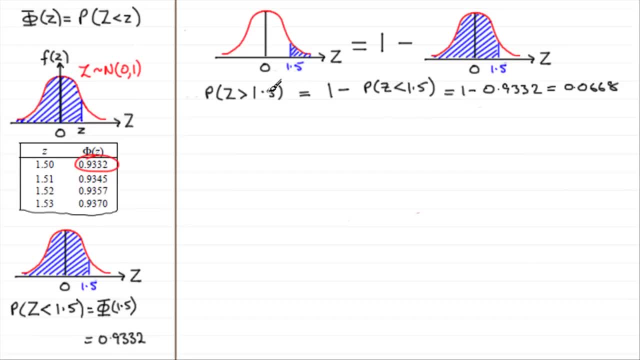 So that's how you can work out the probability of being more than a value when that value is to the right of 0. But that's not always going to be the case. For instance, we could get a question like this: The probability of being more than a negative value. 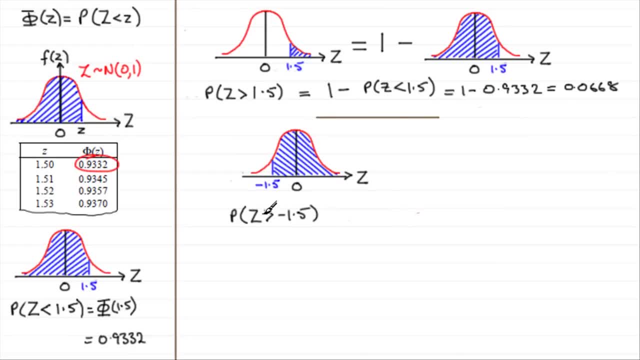 And that's given by this shading. And in this case, the probability of Z is greater than minus 1.5 standard deviations. How do you think we would do that? Well, what we need to do is just use the symmetry of the graph. 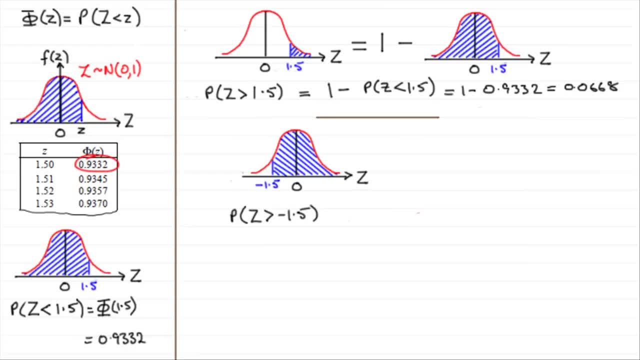 We could reflect this area in the axis And notice here, because the graph is symmetrical, we see that the probability of being more than minus 1.5 is the same as the probability of Z being less than 1.5.. And we've already got that value. 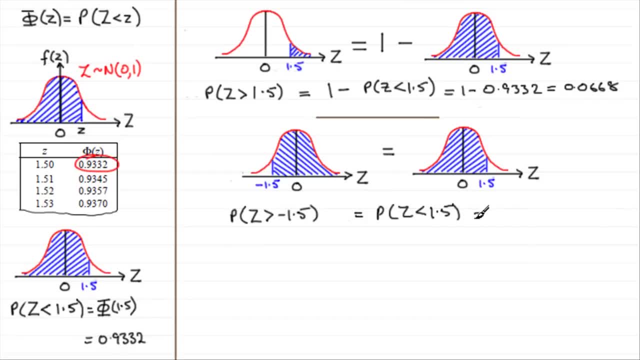 You can see it's 0.9332.. So that's how you would go about working out values that are going to be greater than a negative value. Just reflect that value across the 0, so it becomes the positive value and you're looking at less than. 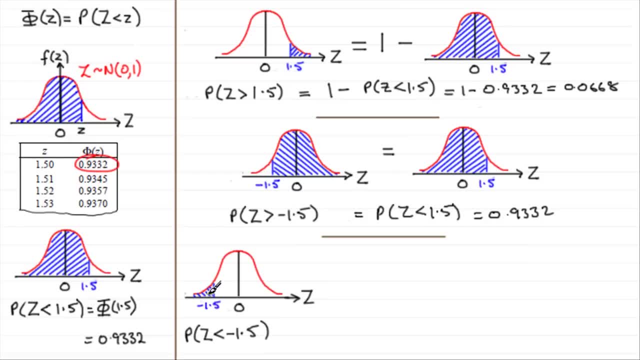 Here's another one. We've got 1.5 standard deviations below the mean. In other words, Z is minus 1.5.. And we want the probability that Z is less than minus 1.5.. So how are we going to work that out?